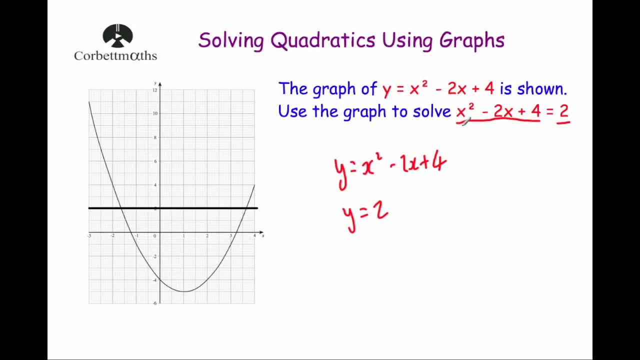 equation. all you need to do is find where those two graphs meet. so you just draw the graph for this and you found where they meet each other. so here you can see they cross here and they cross here, and then you just go down and read off the values on the x-axis and they would be your two solutions. 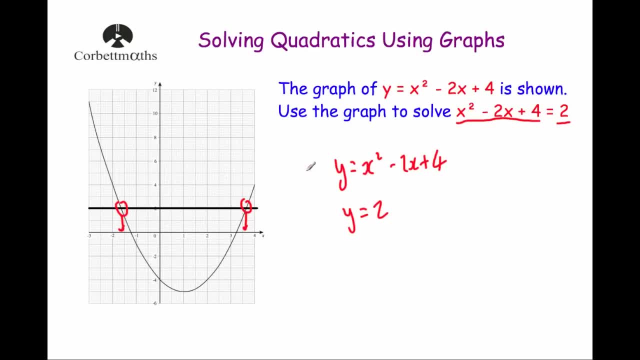 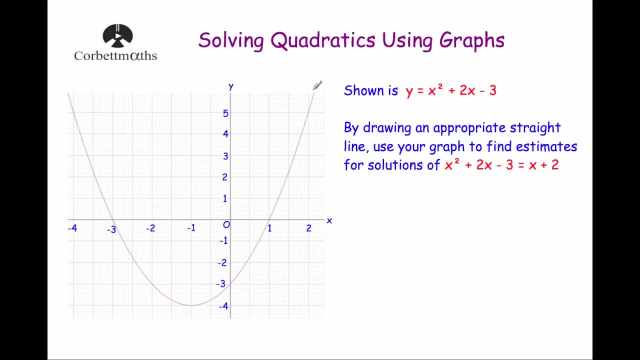 okay, so that's what I covered at the end of the last video. what I'm now going to do is look at some slightly more complex examples. so here's our first example. so we've got the graph, for y equals x squared plus 2x minus 3, and it says: by drawing an appropriate straight line, use your graph to. 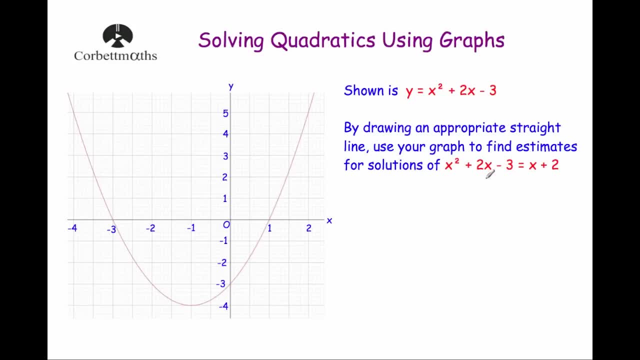 find estimates for the solution. So I'm going to draw a straight line and I'm going to use the solutions of x squared plus 2x minus 3 equals x plus 2. so, as you'll notice, our graph here is y equals x squared plus 2x minus 3, and that's the graph for the expression on the left hand side of 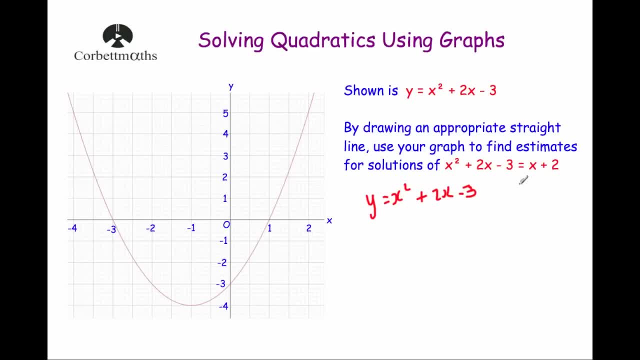 the equation. now what we're going to do is we're going to draw this graph here, the graph of y equals x plus 2, okay so. and when we draw that graph, we find where it meets the quadratic curve, and those point or points will become the solutions. so let's first of all do an xy table, so x y 0, 1, 2, 3, so to find our 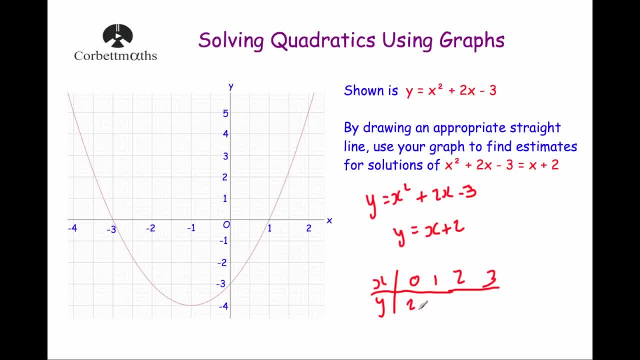 y value. we're just going to add 2 to the x value. so adding 2 gives us 2, adding 2 gives us 3, 4 and 5, and plotting those points would be here: 1, 3, 2, 4. my next point: I should have really have thought. 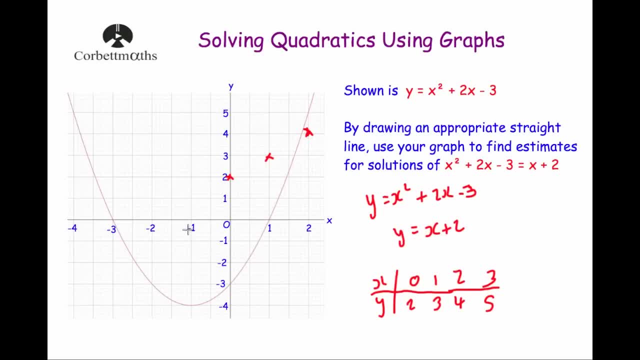 about the graph. but you know, we've got three points anyway, they're all a nice straight line, so we'll just show a line straight through those points. there we go. so that's the graph. the straight line is the graph: y equals x plus 2 and we've got our curve: y equals x squared plus 2x. 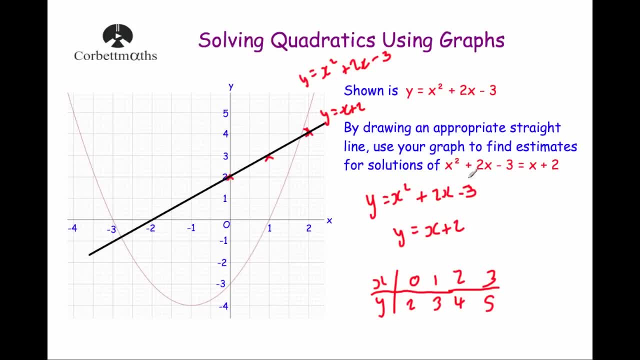 minus 3. so to solve this equation, where you've got x squared plus 2x minus 3 equals x plus 2- we've drawn our graph, our straight line, we've drawn our, we've got our quadratic graph drawn for us. all we need to do is find where they meet each other. so we've got this point here. we've got this point. 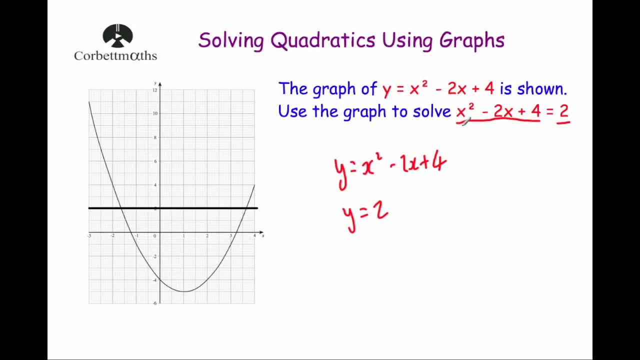 equation. all you need to do is find where those two graphs meet. so you just draw the graph for this and you found where they meet each other. so here you can see they cross here and they cross here, and then you just go down and read off the values on the x-axis and they would be your two solutions. 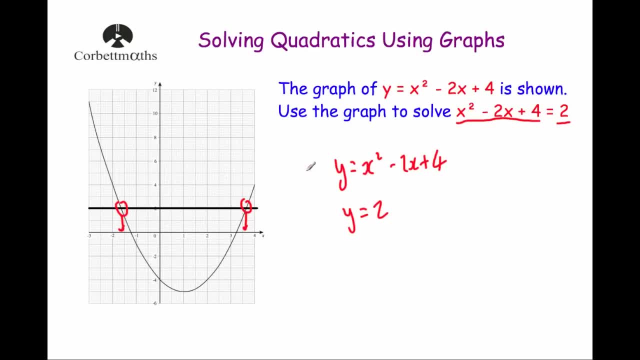 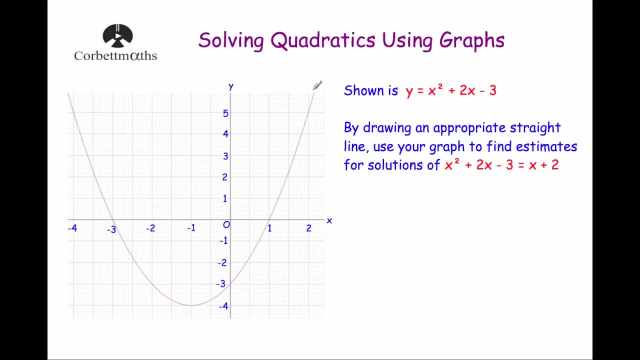 okay, so that's what I covered at the end of the last video. what I'm now going to do is look at some slightly more complex examples. so here's our first example. so we've got the graph, for y equals x squared plus 2x minus 3, and it says: by drawing an appropriate straight line, use your graph to. 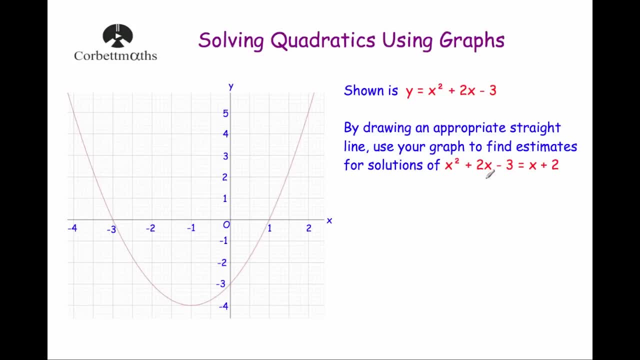 find estimates for the solution. So I'm going to draw an appropriate straight line and I'm going to use the numbers for the solutions of x squared plus 2x minus 3 equals x plus 2. so, as you'll notice, our graph here is: y equals x squared plus 2x minus 3, and that's the graph for the expression on the. 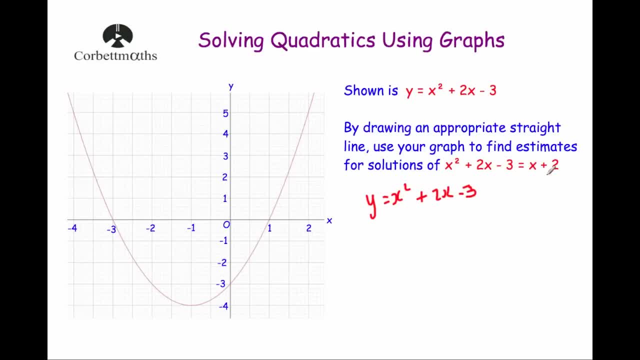 left hand side of the equation. Now, what we're going to do is we're going to draw this graph here. the graph of y equals x plus 2, okay, so, and when we draw that graph, we find where it meets the quadratic curve, and those points are going to be the ones that meet the quadratic curve. So we're. 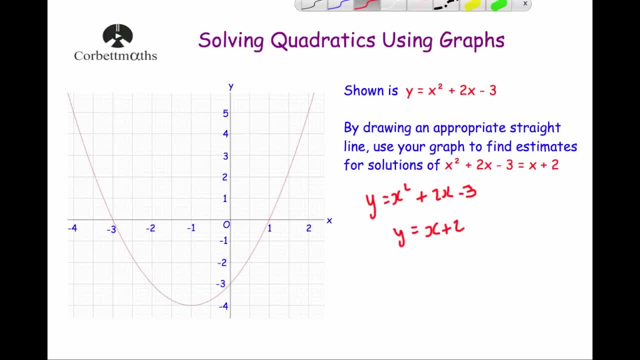 going to call that point a point and these points will become the solutions. So let's first do an x y table. so x y 0, 1, 2, 3, so to find our y value. we're just going to add two to the x value, so 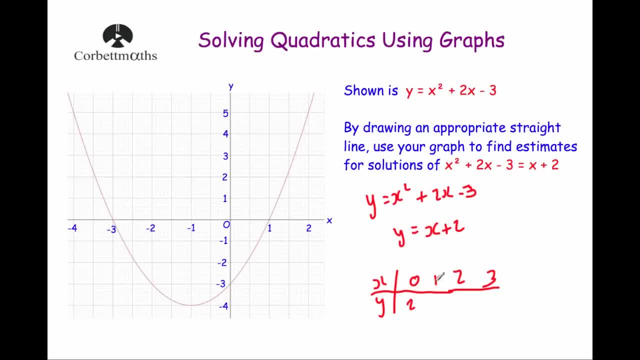 adding 2 gives us 2. adding 2 gives us 3, 4 and 5.. The problem, there are points would be here: 1, 3, 2, 4. my next point- I should have really thought about it- 3, 3 and 4. so there are just 4 points. So let's. 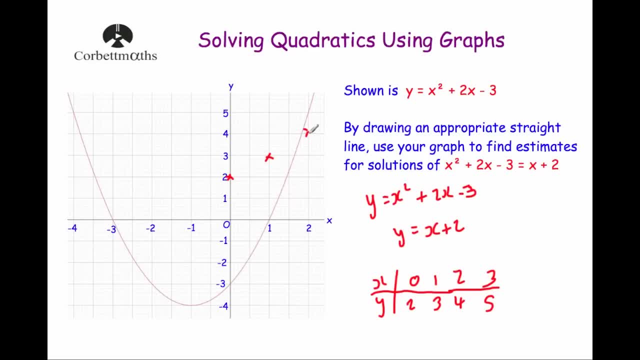 find y and adding y to the x value. Now you see, if we make xys Dak, and now we added y to the x value and zie all be here within three points. this is the problem. and all the points are equal Party. It's not on the graph, but we've got three points anyway and they're all in a nice straight line. 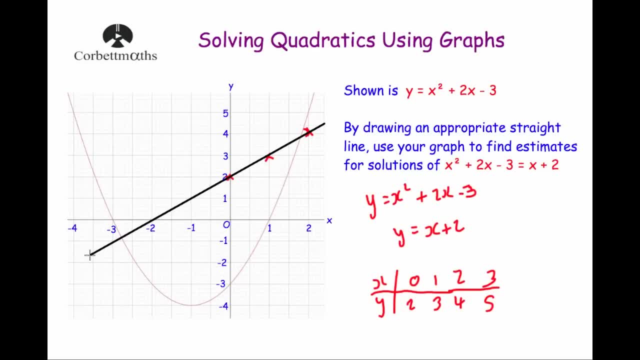 So we'll just show a line straight through those points. There we go. So that's the graph. This straight line is the graph. y equals x plus 2.. And we've got our curve. y equals x squared plus 2x minus 3.. 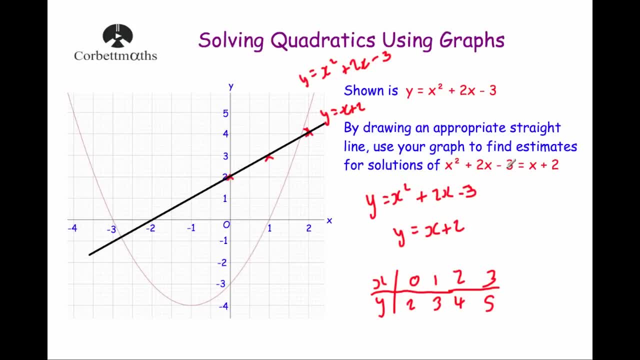 So to solve this equation, where you've got x squared plus 2x minus 3 equals x plus 2, we've drawn our graph, our straight line, We've got our quadratic graph drawn for us. All we need to do is find where they meet each other. 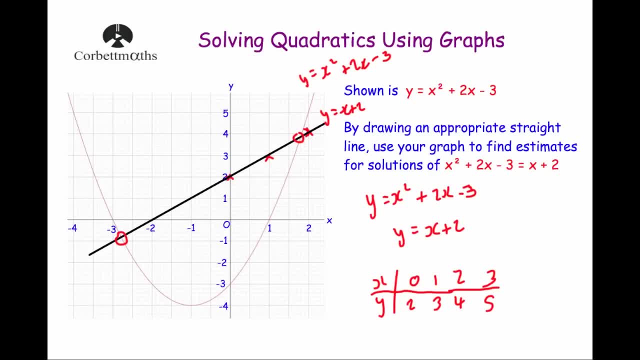 So we've got this point here. We've got this point here. So that's where they meet each other. So we just need to find the x values of those two particular coordinates. So we're going to go up here to that point and we're going to go down from this one to that point. 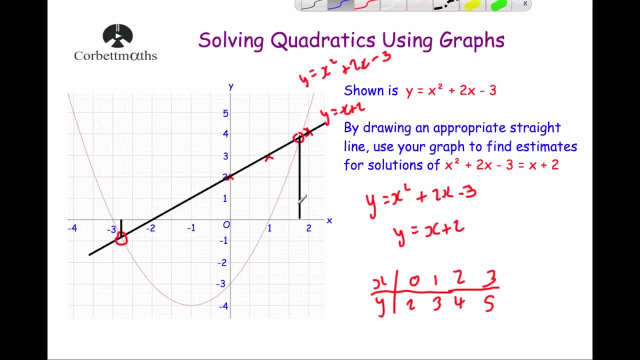 Okay, so our points are: this one here is 1.8, and this one here is minus 2.8.. So our solutions are: x equals minus 2.8.. Or x equals minus or, sorry, x equals 1.8, and that's our two solutions. 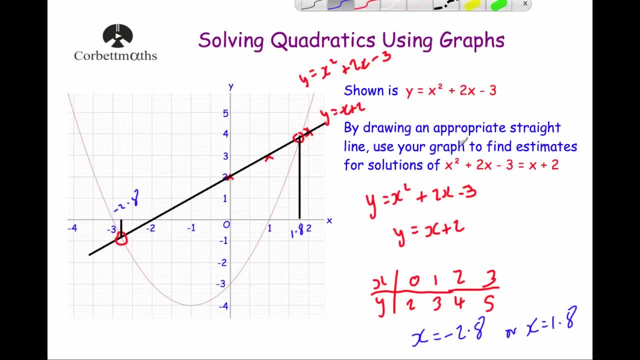 So that's how you do it. If you've got an equation where you've got a quadratic on one side and either a quadratic or linear on the other side, if you draw the two graphs and find where they cross each other, they will be your solutions. 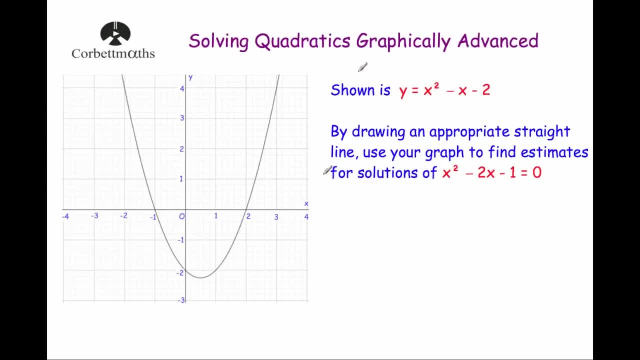 Okay, let's have a look at another example. Right, so let's have a look at our second example. This time, it says, showing us the graph of the curve: y equals x squared minus x minus 2.. And it says, By drawing an appropriate straight line: 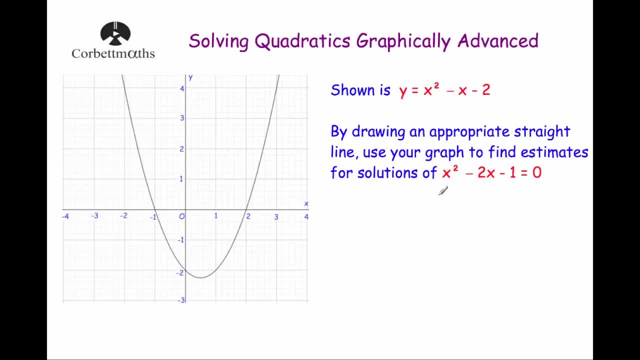 you use your graph to find estimates for the solutions of x. squared minus 2x minus 1 equals 0.. Now, as you notice this, the graph we've been given is completely different to the expression on the left-hand side of the equation. 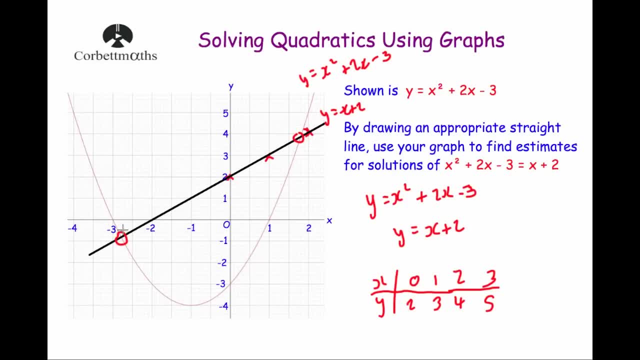 here. so that's where they meet each other. so we just need to find the x values of those two particular coordinates. so we're going to go up here to that point and we're going to go down from this one to that point. okay, so our points are: this one here is 1.8 and this one here is minus 2.8. so 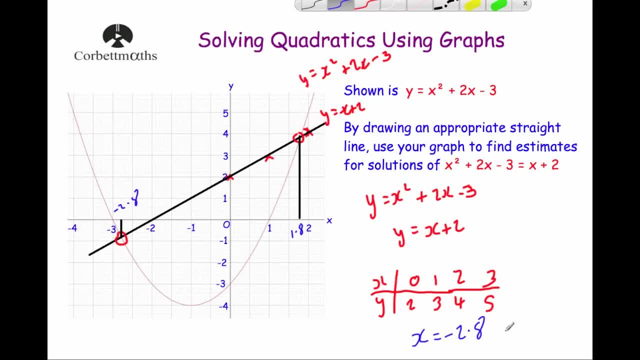 our solutions are: x equals minus 2.8, or x equals minus or, sorry, x equals 1.8, and that's our two solutions. so that's how you do if you've got an equation where you've got a quadratic on one side and either a quadratic. 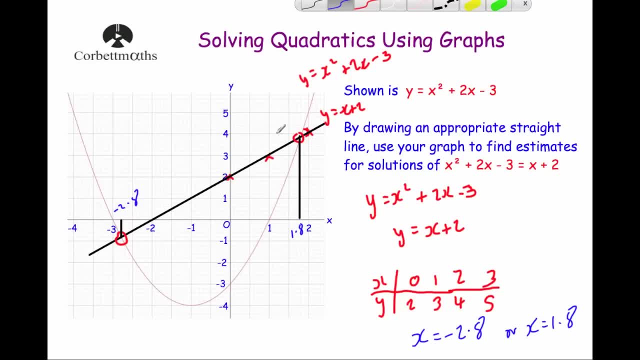 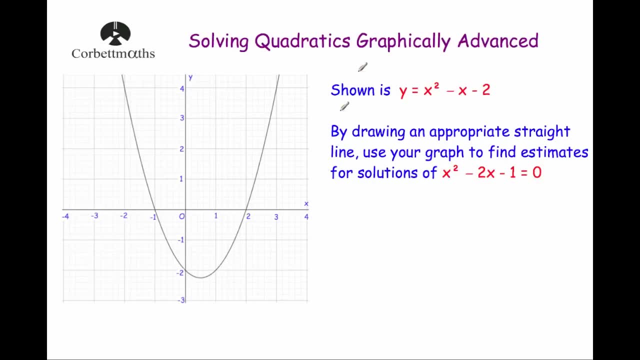 or linear. on the other side, if you draw the two graphs and find where they cross each other and they will be your solutions. okay, let's have a look at another example. all right, so let's have a look at our second example. this time it says: shown is the graph of the curve. y equals x squared minus. 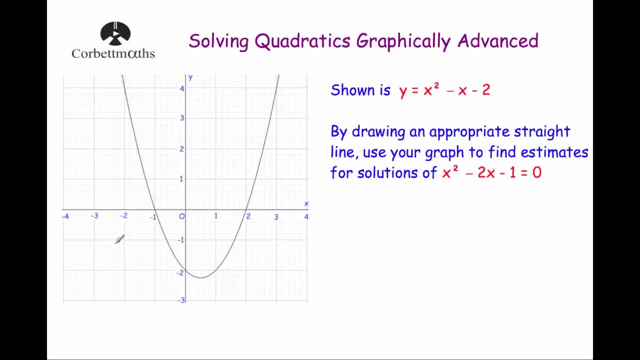 x minus two, and it says: by drawing an appropriate straight line, use your graph to find estimates for the solutions of x squared minus two. x minus one equals zero. now, as you notice, this um the graph we've been given is completely different to the expression on the left hand side of the equation. so what we're going to do is we're going to consider our 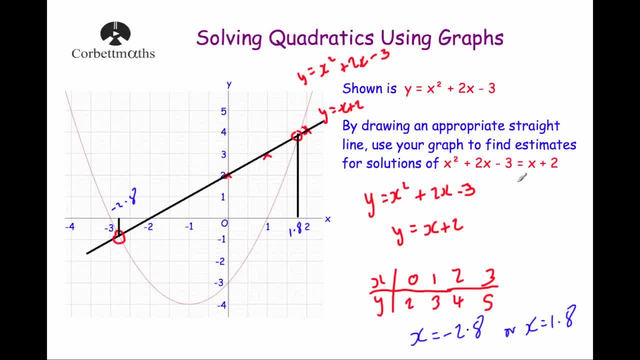 last example and our last example: the equation that we had to solve and the actual curve we've been given. they're both, um, obviously the same. we had our x squared plus two x minus three, x squared plus two x minus three. now what we're going to do is we're actually going to use this, okay. 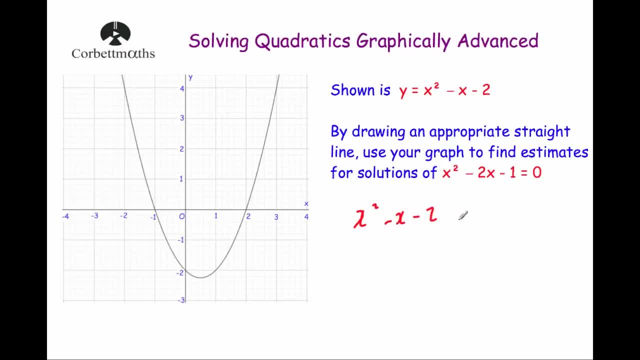 our x squared minus x minus two. okay, now what we're going to do is we're going to put it equal to something. okay, because, as we see, our equation is x squared minus two, x minus one. now, if we had something here and we took it away from both sides, we could end up with this equation here. 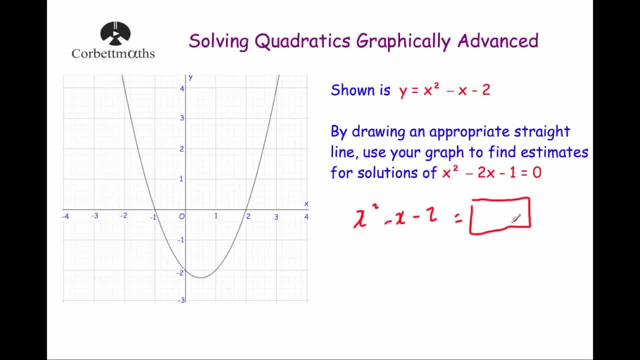 okay. so we just need to figure out what would be here, so that if we took it away from both sides, we would get to x squared minus two. x minus one equals zero. okay now, as you can see here, we've got minus x and then it goes to minus two x. that means we're going to be taken away in over x. 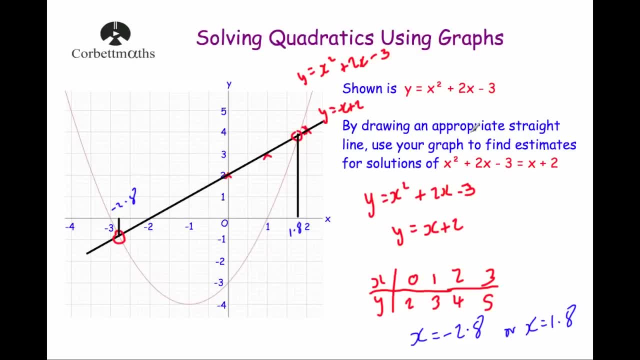 So what we're going to do is we're going to consider our last example. and our last example, the equation that we had to solve and the actual curve we've been given. they're both obviously the same. We had our x squared plus 2x minus 3, x squared plus 2x minus 3.. 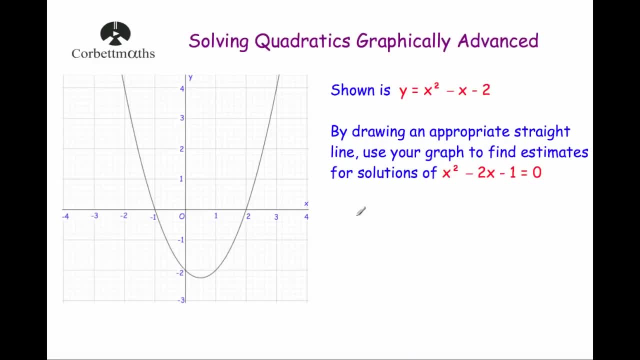 Now, what we're going to do is we're actually going to use this: okay, our x squared minus x minus 2, okay, Now, what we're going to do is we're going to put equal to something. okay, Because, as we see, our equation is x squared minus 2x minus 1.. 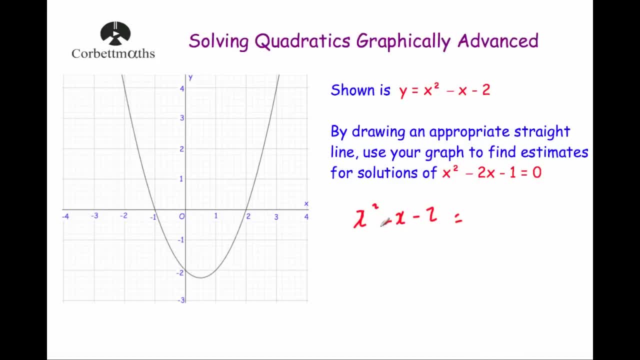 Now, if we had something here and we took it away from both sides, we could end up with this equation here: okay, So we just need to figure out what would be here so that if we took it away from both sides, we would get to: x squared minus 2x minus 1 equals 0, okay. 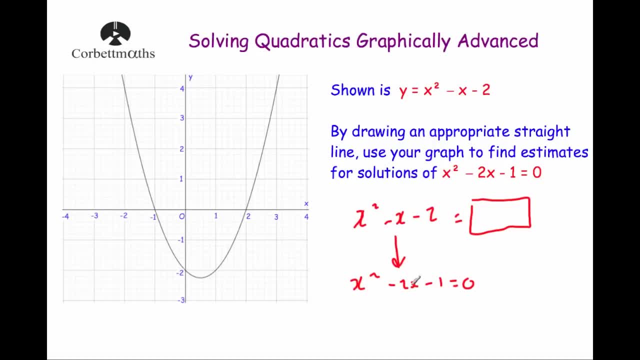 Now, as you can see here, we've got minus x and then it goes to minus 2x. That means we're going to be taking away another x. We're going to be taking away an x to get from here to here. 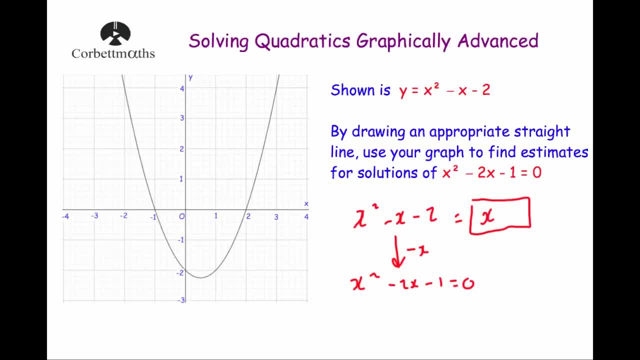 and that means that if we have an x on the sides of the equation, that means that we would have an x on the set of the equation, So that we would take it away from both sides to get 0, okay, So what else have we got? 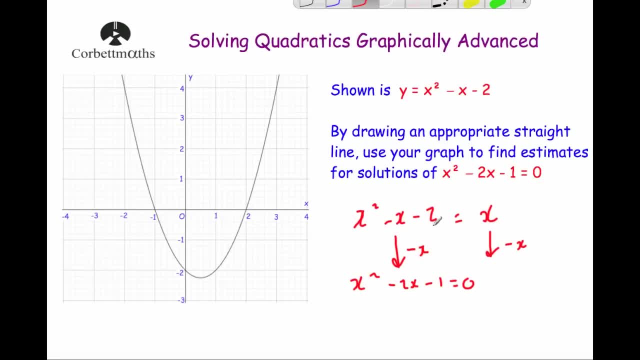 We've got a number okay because, as you can see here, we've got minus 2, and we need to get to minus 1.. Okay one. Then you get from minus two to minus one. you actually add one, Okay. So that means that. 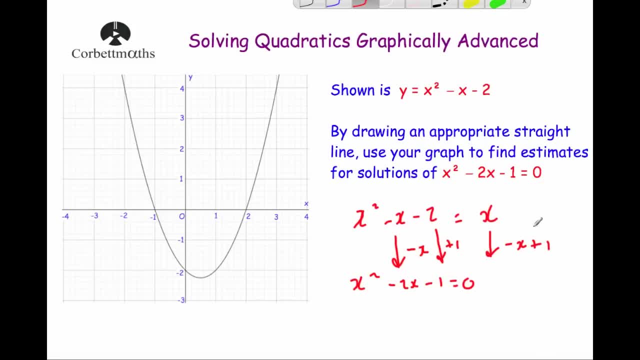 we're going to need to add one to both sides of the equation. Now, if we're adding one to both sides of the equation, that means that it's going to have to be a minus one here, because if you add one to minus one you get zero. So if we had x squared minus x minus two equals x minus one. 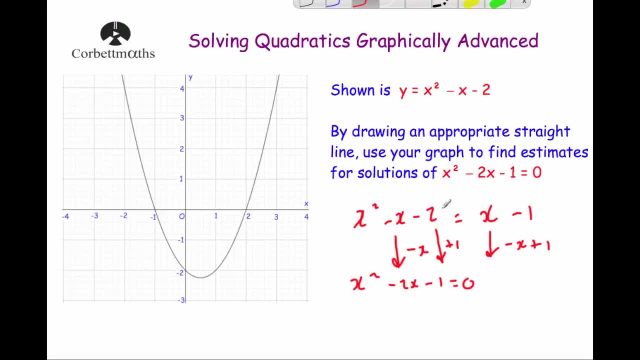 you've got the graph we've been given on the left hand side of the equation, We've got a straight line we can draw And we also know that if we take this x minus, or if we take away x from both sides of the equation and we add one to both sides of the equation, you get the same equation that we. 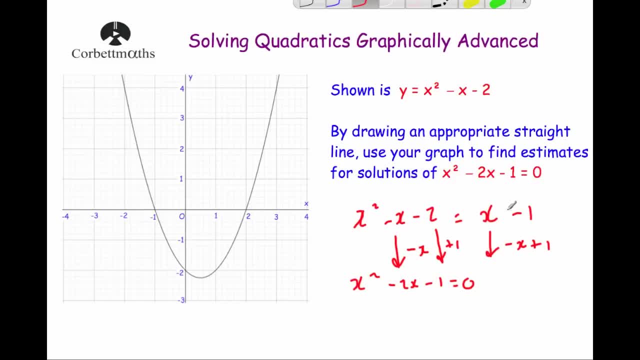 want to solve. Okay, So let's draw this graph: our x minus one. So we're going to draw: y equals x minus one. Done a little: x, y table x, y zero one, two. We're going to take away one from all. 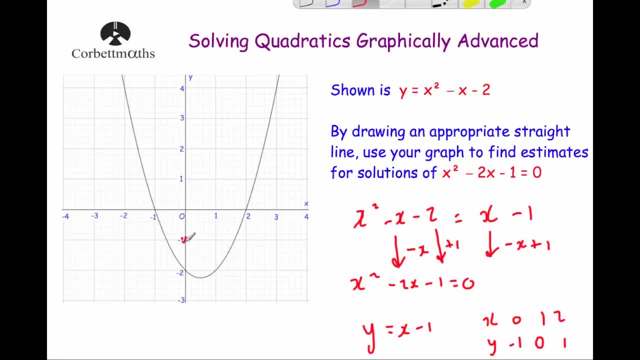 of them, So minus one, zero and one. So plotting those zero minus one one, zero two, one, And we just draw a straight line through them And we find where they meet each other. So they meet here. 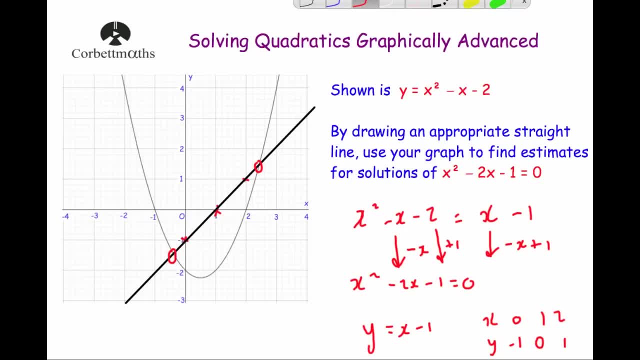 and they meet here. We just need to see what points they are. So if we draw a line straight down here, a line straight up here, we'll get our points. So we've got here. what are these going up in? They're going up in 0.2s, So it's going to be 2.4.. And this one: they're going down in 0.2s. 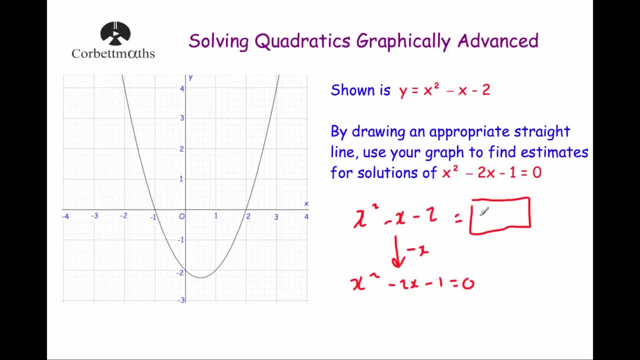 we're going to be taken away in x to get from here to here. now that means that if we have an x on this side of the equation, that means that we would have an x on this side of the equation so that we would take it away from both sides to get zero. okay. so what else have we got? we've got a number, okay. 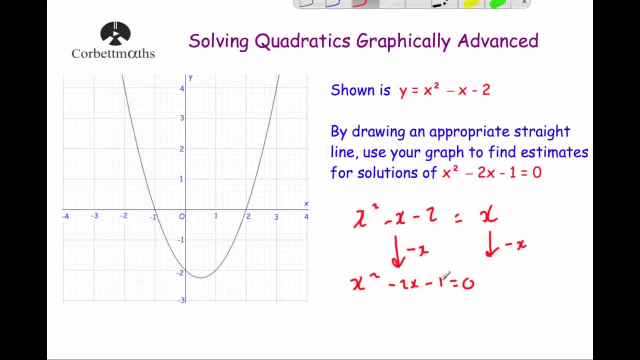 because, as you can see here, we've got minus two and we need to get to minus one. now you get from minus two to minus one. you actually add one, okay. so that means that we're going to need to add one to both sides of the equation. now, if we're adding one to both sides of the equation, that means that 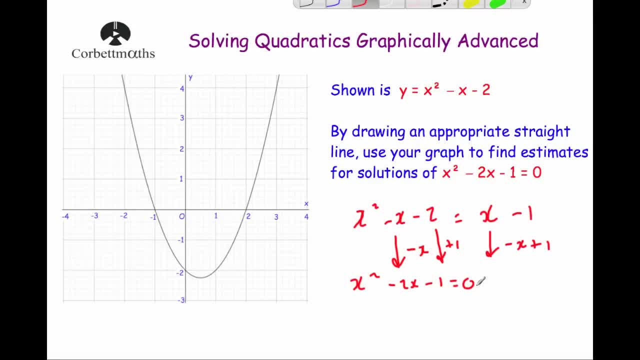 it's going to have to be a minus one here, because if you add one to minus one you get zero. so if we had x squared minus x minus two equals x minus one. you've got the graph we've been given on the left hand side of the equation. we've got a straight line we can draw, and we also know that if we take 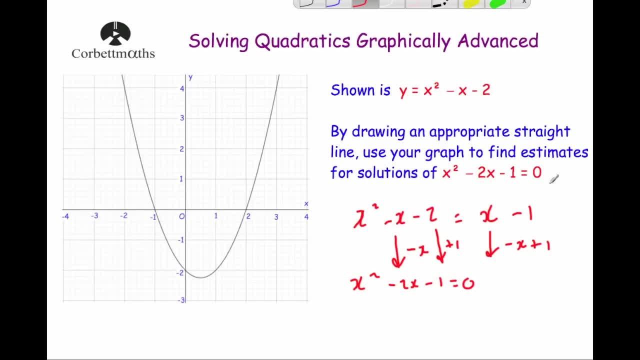 take away x from both sides of the equation and we add one to both sides of the equation, you get the same equation that we want to solve. okay, so let's draw this graph: our x minus one. so we're going to draw: y equals x minus one. done a little, x y table, x, y zero, one, two. we're going to take: 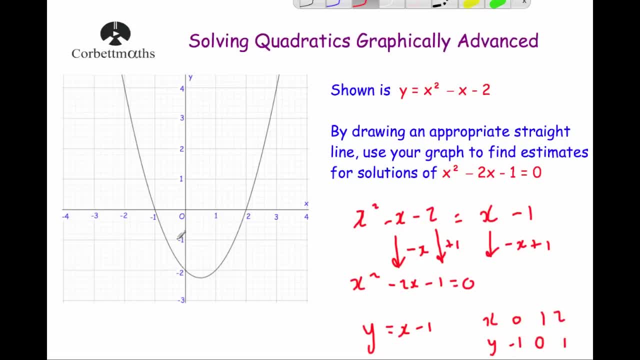 away one from all of them. so minus one, zero and one. so plotting those zero, minus one one, zero two, one, and we just draw a straight line through them and we find where they meet each other. so they meet here and they meet here. we just need to see. 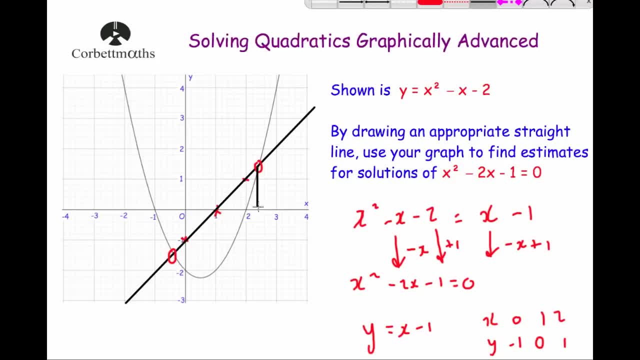 what points they are. so if we draw a line straight down here, a line straight up here, we'll get our points. so we've got here. what are these going up in? they're going up in 0.2, so it's going to be 2.4. and this one: they're going down in 0.2, so it's. 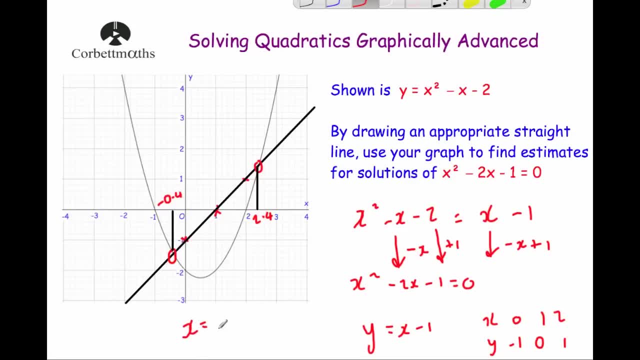 going to be minus 0.4, and that's our solutions: x equals minus 0.4 or x equals 2.4. okay, so the main thing is, if you've been given a quadratic graph or y equals, and you've got an equation you need to solve by using an appropriate straight. 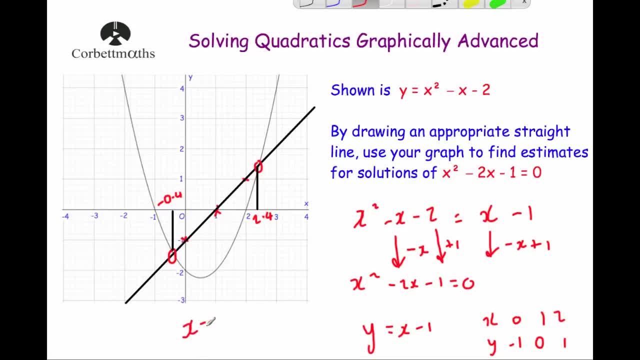 It's going to be minus 0.4.. And so solutions: x equals minus 0.4, or x equals 2.4.. Okay, So the main thing is if you've been given a quadratic graph, or y equals, and you've got an equation that you need to solve, 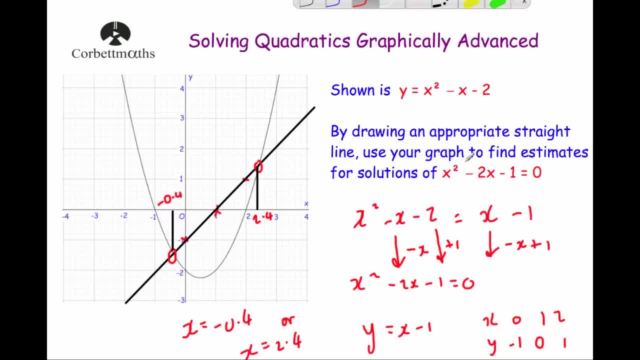 by using an appropriate straight line, and it doesn't clearly equal that. what you can do is find out what the linear would be on the other side, or even possibly a quadratic, and you could draw that. Okay, let's have a look at another example, just to go through it again. So here, 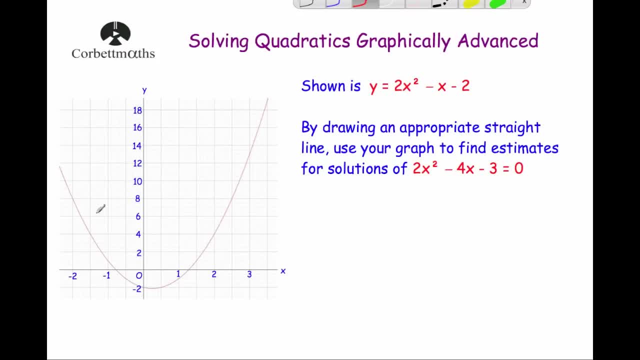 we've got the graph: y equals 2x squared minus x minus 2.. And it says: by drawing an appropriate straight line, use your graph to find the estimates for the solutions of 2x squared minus 4x minus 3 equals 0.. Now 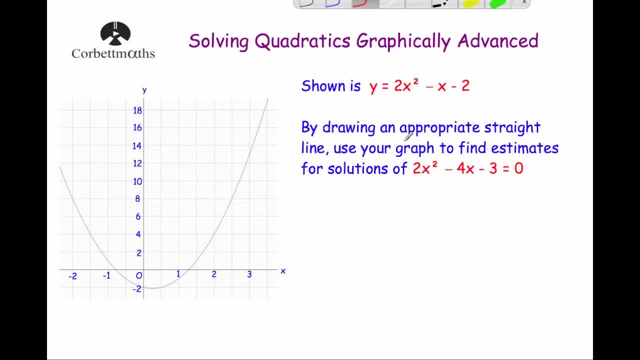 clearly, this quadratic is not the same as this quadratic here. Okay, So what we're going to do is we're going to, we're going to write this: 2x squared minus x minus 2. And it's going to equal something. It's going to equal a linear expression, a straight line, something x and a number. 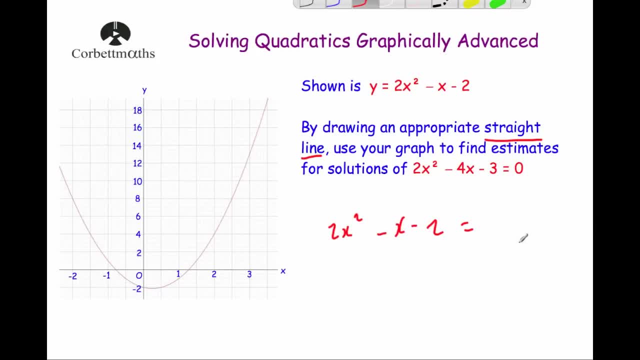 And it's whenever we take it away or add it to both sides, we're going to get to our 2x squared minus 4x minus 3 equals 0. So we just need to think how we get from here to here. here to here. 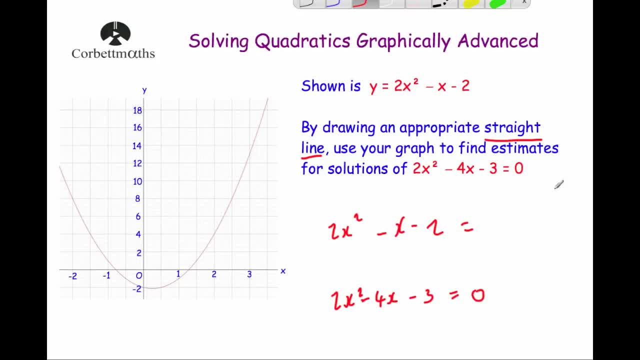 and that would help us work out what this expression will be on the right-hand side of the equation. So to get from minus x to minus 4x, we would take away three x's. Now if you're taking away three x's from both sides of the equation, that means that it's going to have to. 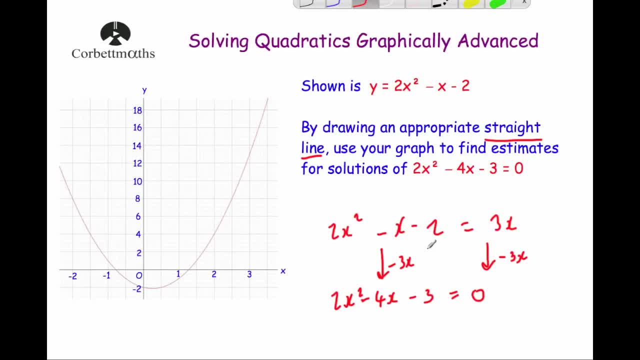 be a plus one. And next, to get from minus 2 to minus 3, you take away one. So that means that you're going to be taking away one from both sides of the equation, So that means that must be a plus. 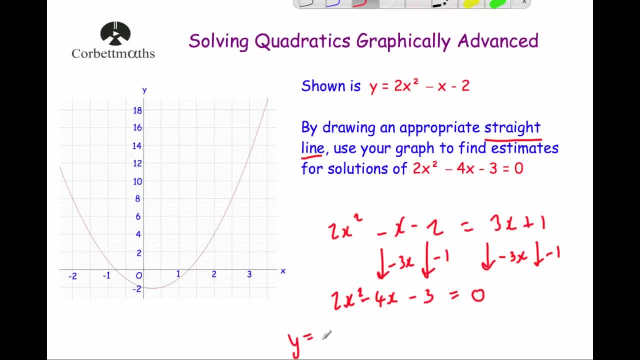 one. So the straight line graph we're going to draw is: y equals 3x plus 1.. So let's draw that graph xy, table xy: 0, 1,, 2, times about 3, add 1, 1, times about 3, add 1, 4, times about 3, add 1, 7.. 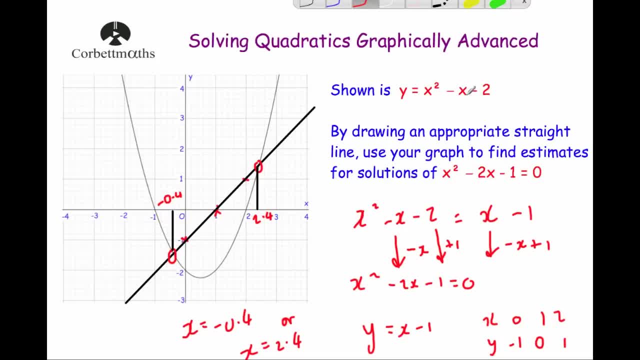 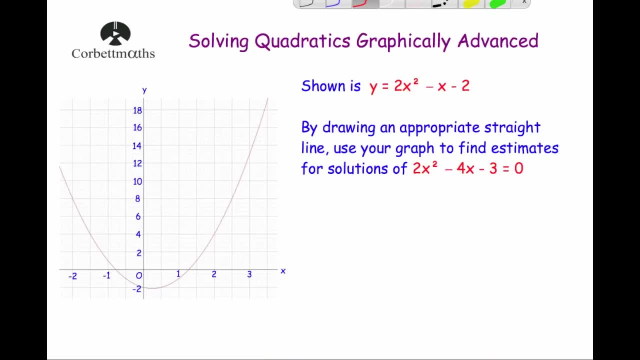 line and it doesn't clearly equal that. what you can do is find out what the linear would be on the other side, or even possibly a quadratic, and you could draw that. okay, let's have a look at another example, just to go through it again. so here we've got the graph. y equals 2x squared. 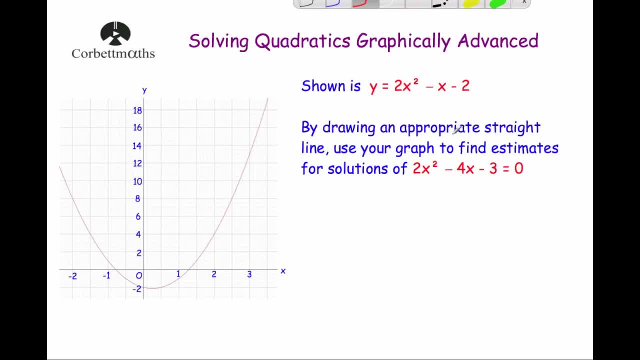 minus x, minus 2, and it says: by drawing an appropriate straight line, use your graph to find the estimates for the solutions of 2x squared minus 4x minus 3 equals 0.. now, clearly, this quadratic is not the same as this quadratic here. 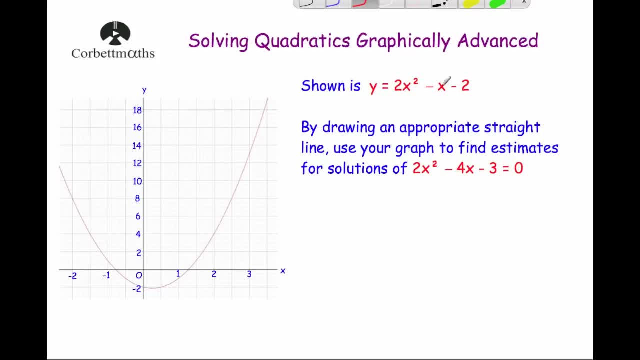 okay. so what we're going to do is we're going to, we're going to write this: 2x squared minus x minus 2, and it's going to equal something. it's going to equal a linear expression, straight line, a, something, x and a number, and it's whenever we take it away or add it to both sides, we're going to get. 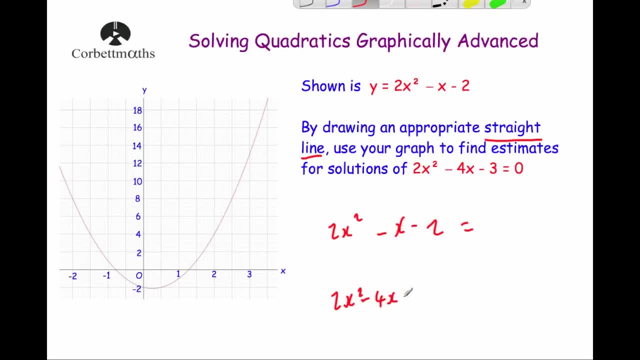 2x squared minus 4x minus 3 equals 0.. so we just need to think how we get from here to here, here to here, and that would help us work out what this expression will be on the right hand side of the equation. so to get from minus x to minus 4x, we would take away three x's. now, if you're taking 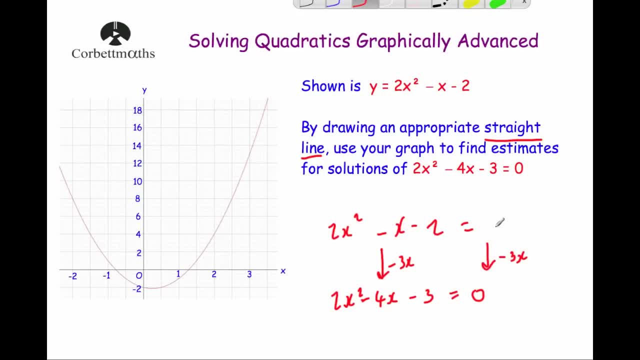 away three x's from both sides of the equation. that means that it's going to have to be a 3x here and next to get from minus 2 to minus 3, you take away one. so that means that you're going to be taking away one from both sides of the equation. so that means 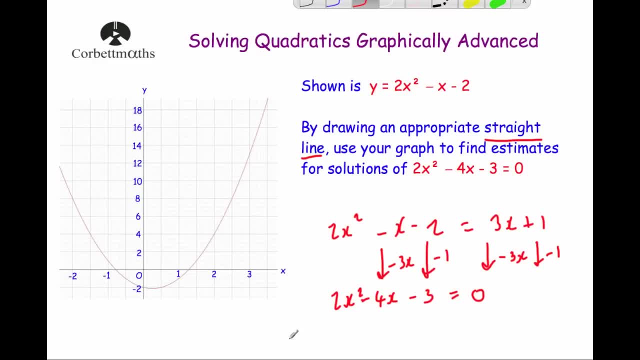 that must be a plus one. so the straight line graph we're going to draw is: y equals three x plus one. so let's draw that graph: uh x, y. table x: y. zero one two times about three. add one one times about three. add one four times about three. add one seven. so zero one, uh, one, four and. 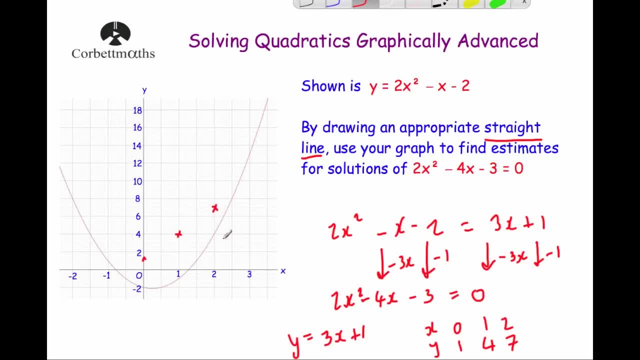 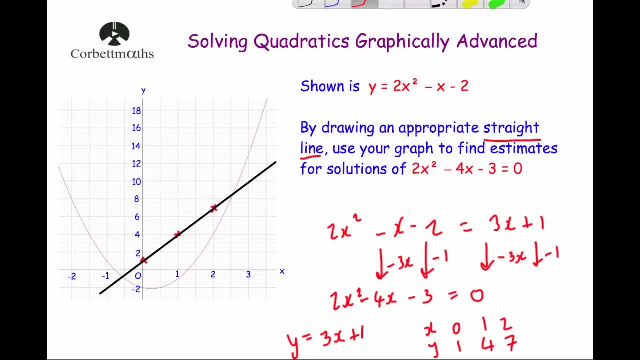 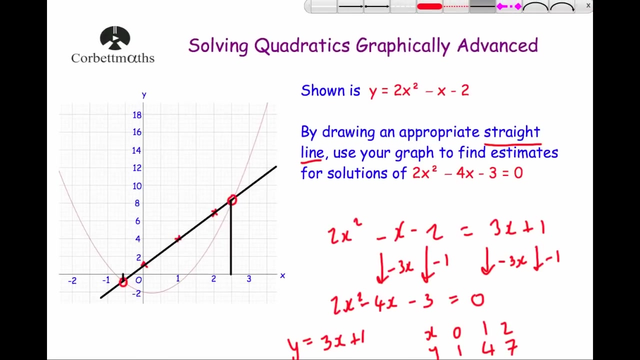 two, seven, okay, and we're going to draw a nice straight line through those, okay, and to then find our solutions, our approximate solutions or estimates for the solutions. we just find where they meet each other. so they cross here and here and we go down, we go up and we get our solutions, which are 2.5 and minus. 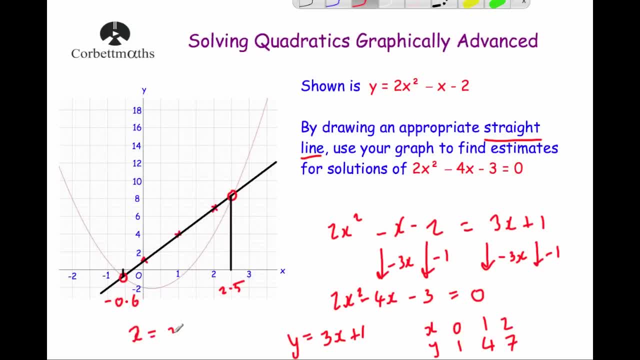 0.6. so x equals minus 0.6, or x equals 2.5, and that's it. 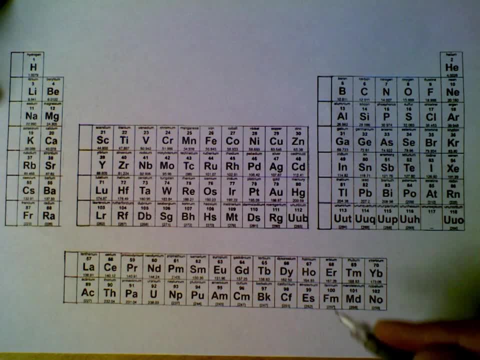 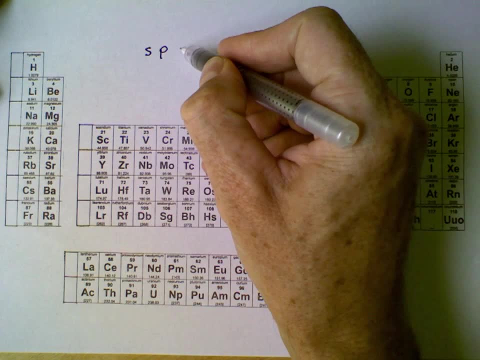 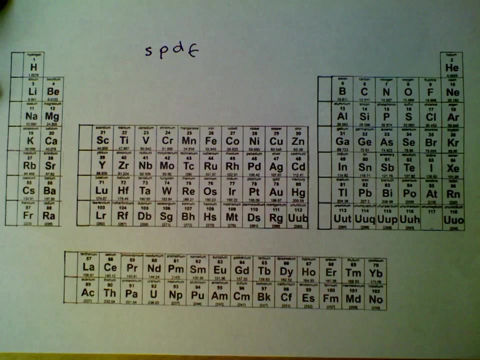 How to prepare your periodic table for quantum mechanics questions. Well, remember, hopefully, that the order of orbital types are S, P, D and then F, And we take our periodic table and we start on the far left hand side with 1, we number downwards. 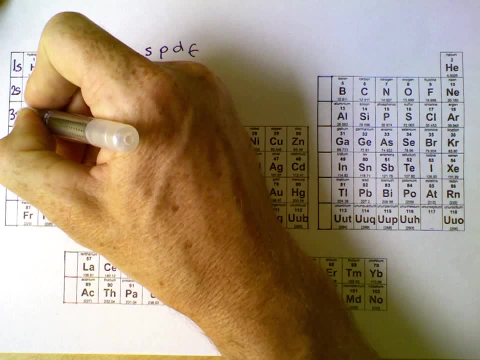 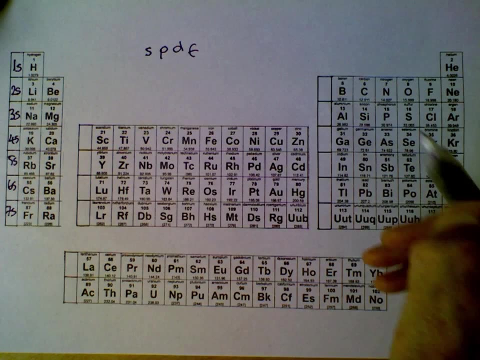 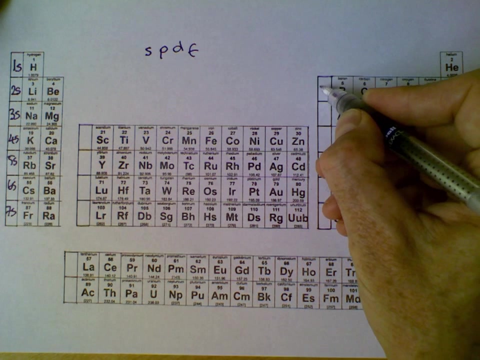 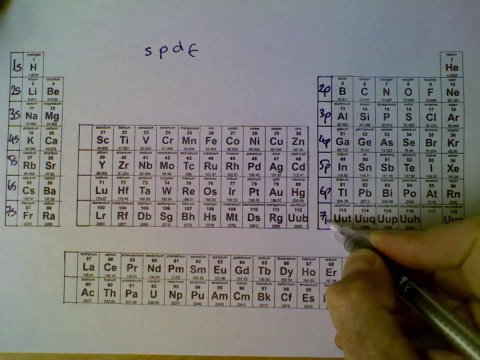 1S, 2S, 3S, 4S, 5S, 6S and 7S. We then move to the next columns along the next taller set of columns, And those are P's and those begin with 2.. So we number these: 2P, 3P, 4P, 5P, 6P and 7P. 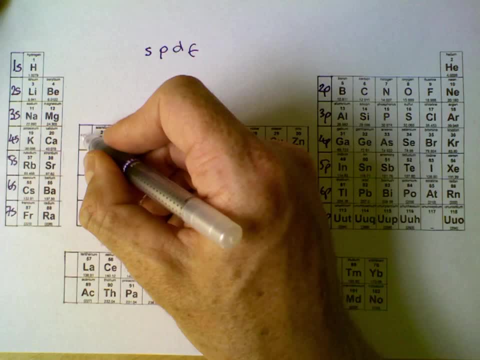 The next column are the D's and they start with 3.. 3P, 4P, 5P, 6P and 7P. 3D, 4D, 5D, 6D. 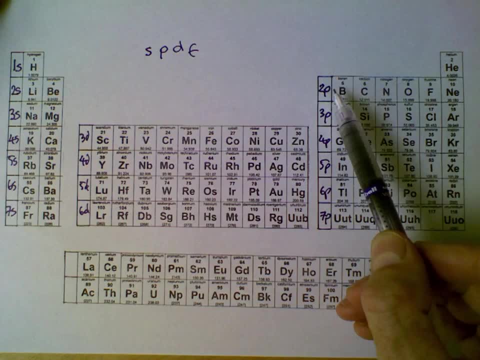 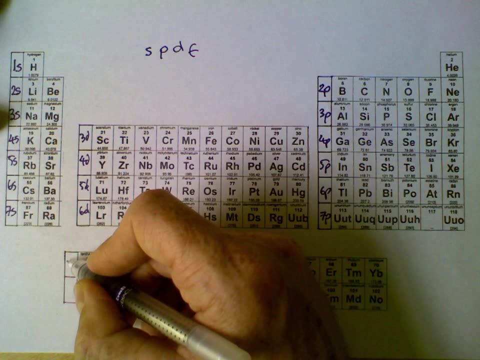 Hopefully you're noticing a pattern: S's starting with 1s, P's starting with 2s, D's starting with 3s And we finish up with F's, starting with 4F Here and 5F here. 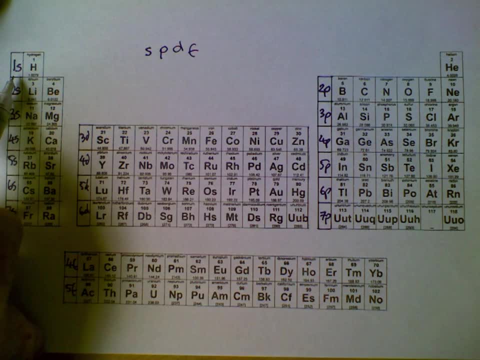 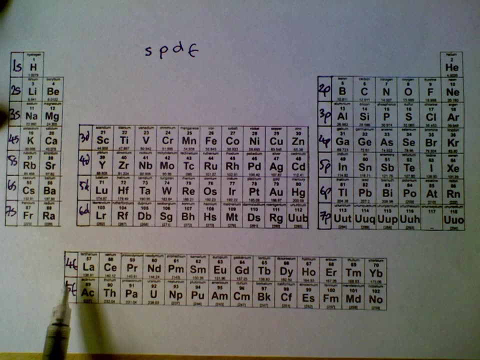 So the order goes: Start with S's begin with number 1. And P's with number 2., D's starting with number 3. And F's starting with number 4..